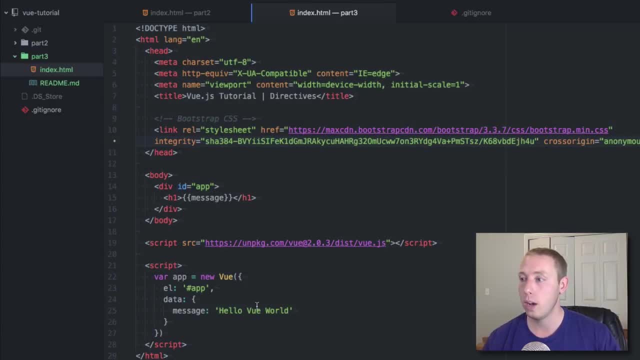 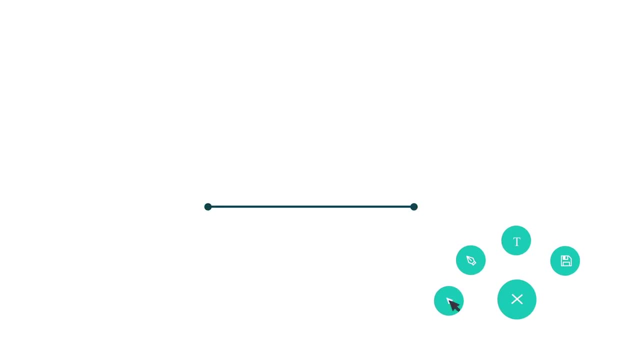 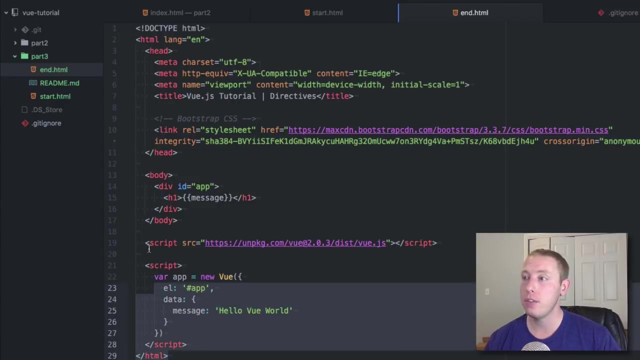 off on part number two. That's what we're going to start with, So let's go ahead and do it. All right, so I'm going to be working again. if you download the source code, you're going to want to start at the starthtml. That will give you the source code that we're basically looking at right here. It's the starting point, so that way you can download the source code, Use the starthtml. 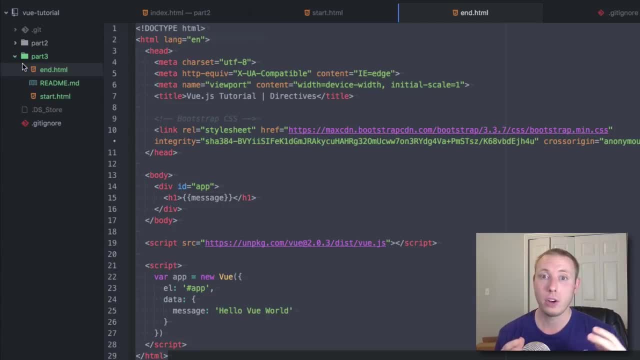 inside of part number three folder and then you're going to basically start the same place that I'm starting, So you have the same code that I have from the beginning. If you want to skip and see what the end result is, you can look at the endhtml, and that's what I'm going to be working on here. 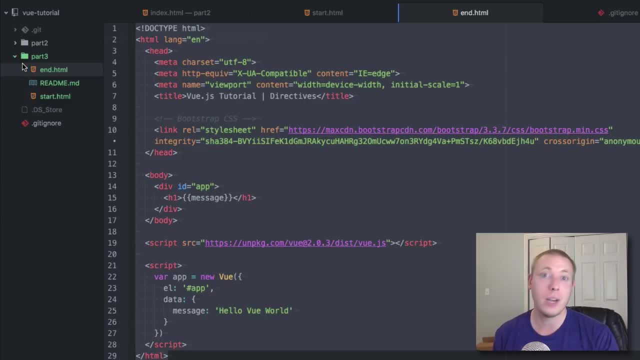 today, but that's basically going to represent the ending of this video here. So all right. so the starthtml is the beginning of the video. The endhtml is the end of the video. So, depending on whether you want the code that I started with or the code that ended at the end of the video, you 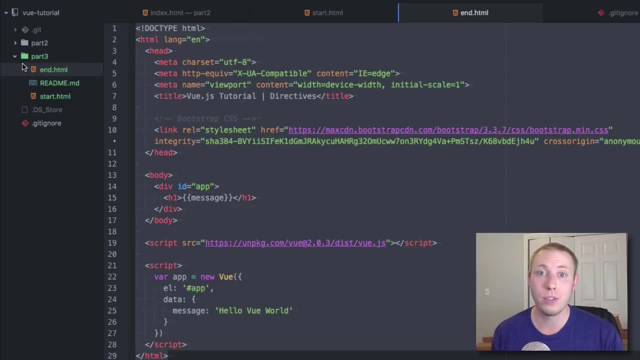 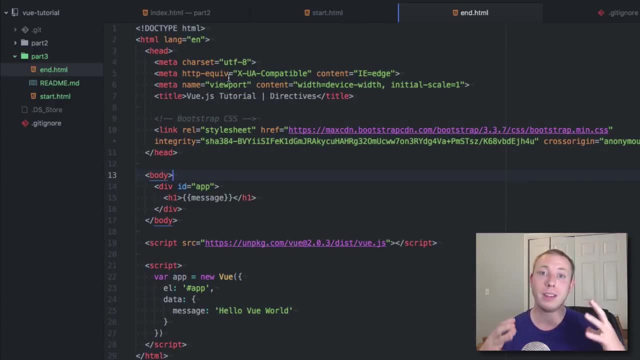 get the appropriate thing. Okay, just want to clarify that. that's how all the future videos in this series will be as well. Okay, and it's all inside of the folder for that video part. Okay, now let's talk about what we're talking about today, which is these directives- Now directives. 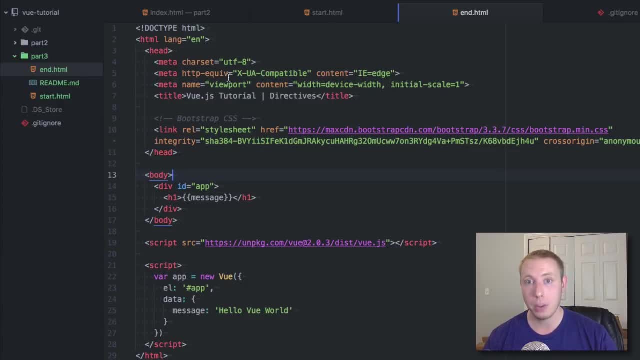 in Vue are really, really handy. They go right in line with our divs, similar to any other attribute that you might be used to in html, and they're all represented with the v dash prefix, basically. So let me give you an example of what, of basically what a directive is, And remember, directives are like common functionality that you 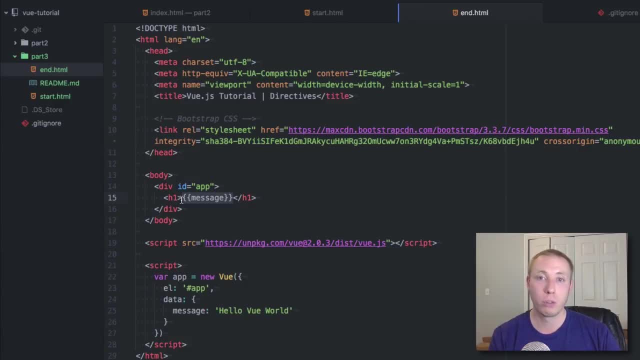 use over and over again. They're like mini functions, but you can throw them right in line in your div, So let me give you a quick example. So, first of all, we can go here and we can see. this is again where we picked up in the last video. I'm going to show you the first directive. 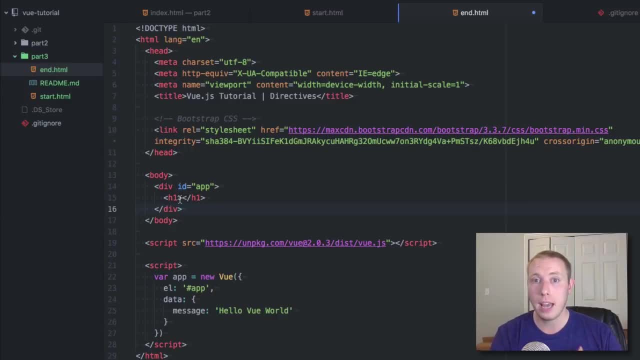 which is called v text. Now, v text simply adds text to whatever element you you're adding the v text to. Okay, so let me show you how it works. We're going to add that message, just like we did in the last video, but instead of doing mustache brackets, we're going. 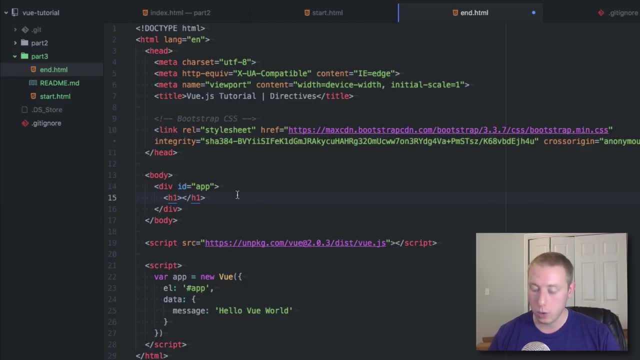 to use the v text directive. Okay, so let's go over here to h1.. Let's give it a little space here and we're going to do v? dash text and we're going to do v? dash text and we're going to set it equals. 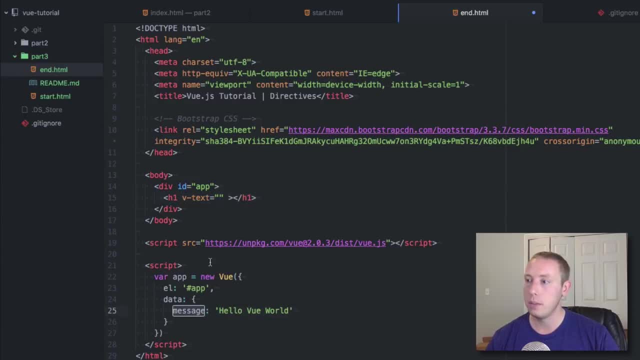 to our equal to message Okay, so let's go ahead and do that message. We're going to go and click save and I don't need to add my message in here right now. We're just going to do the v text and again, all of these directives are prefixed with the v dash Okay, and the v? dash text, just. 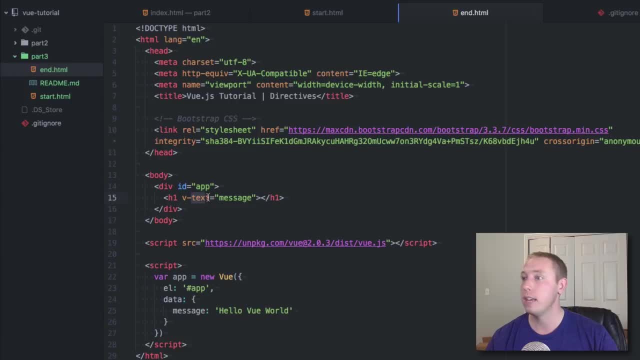 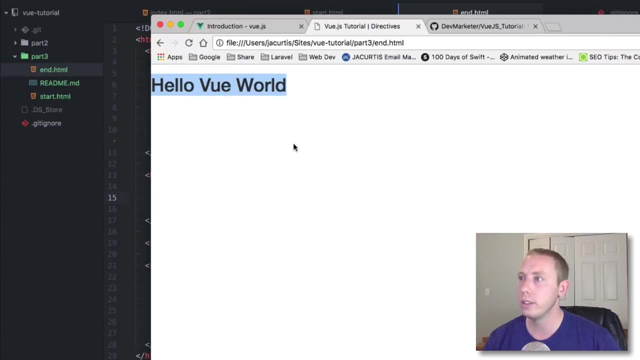 simply says: add this text to this element. Pretty basic. Let's go ahead and save it. and now let's open this in the browser. Okay, so now, as you can see in the browser here, we get the exact same thing. It says: hello, view world. and again, if we do the same thing we did in the last video, let's go. 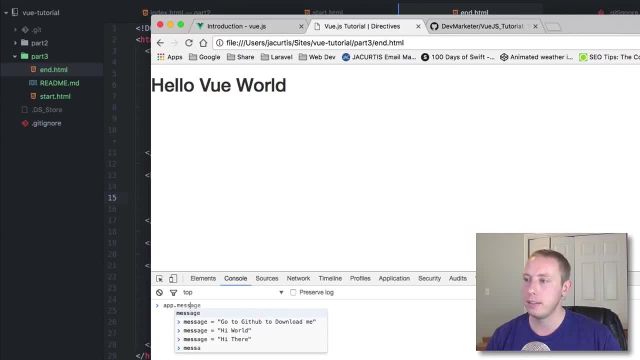 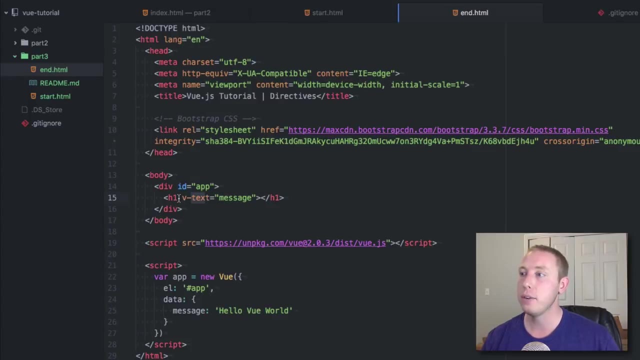 over to our console and let's just change appmessage and set it equal to go dev marketer, And we click enter and you can see it's binding in exactly the same way as it did before. The difference now is, though, we use this directive to place it instead of the mustache brackets. Okay, 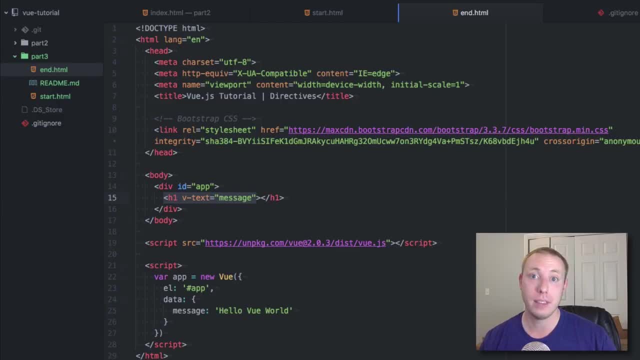 so that just kind of gives you an idea for kind of some of the stuff that this does. Now let's take a look at a couple of the other directives that you might want to use, depending on the situation, and we'll talk about some of the advanced ones at the end. So another one you can use in addition to v. 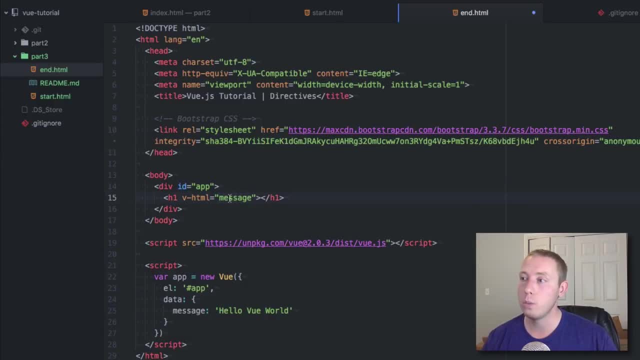 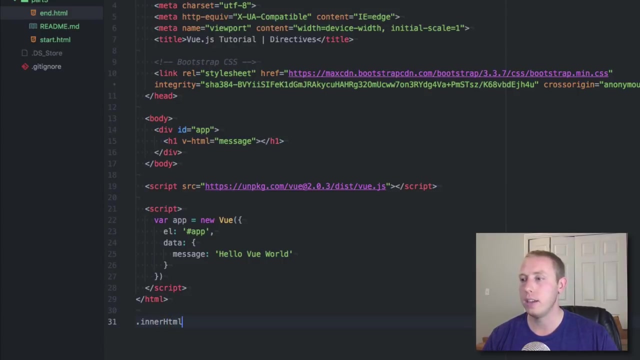 text is v html, It does the exact same thing as v text. It inserts this into this element, but it will insert actual html, It won't. it's like the inner html attribute, So you might be familiar with. if you did something like in javascript, you'd use this dot inner html- Is it dot inner html? like that, and you could insert. 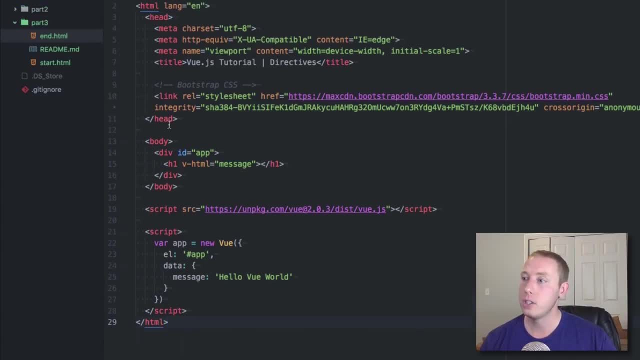 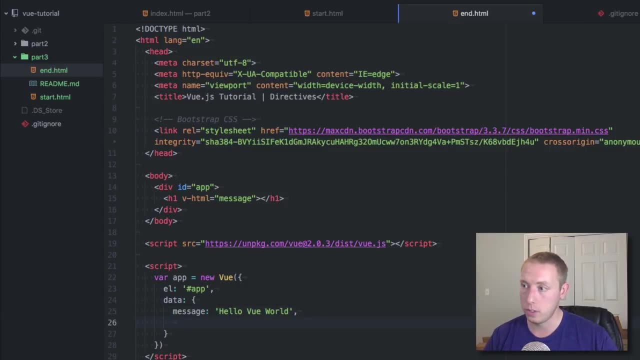 html inside of an element. That's basically what this does. All right, so we do v? html and then we're going to add message. What we can do here is add another- you know data set actually- and we'll say: we'll do an intro and what we're going to do is we're going to insert html in here. So we're going to say: 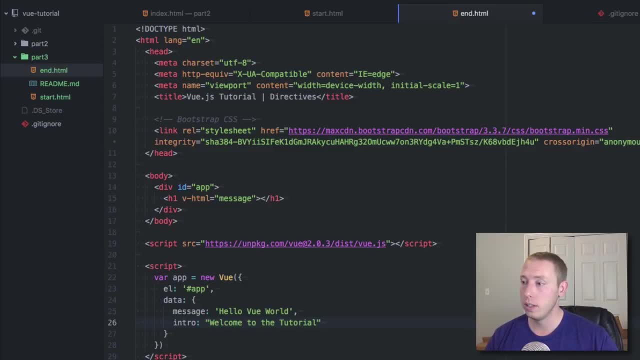 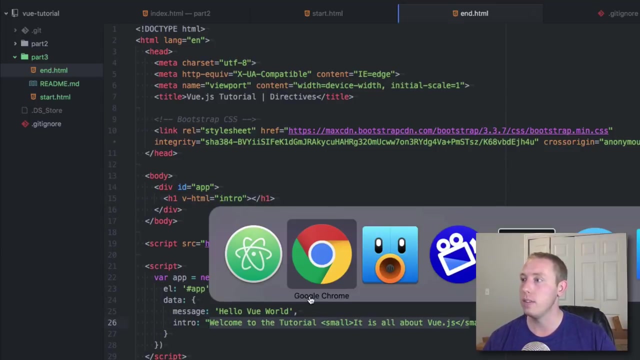 welcome to the tutorial. but then we're going to add this small attribute and this is something an html attribute, and we'll just say it is all about viewjs. Okay, so now this is actually this string here includes html and with this vh html let's change this to intro and it should now pair with this. So let's go and save this move back. 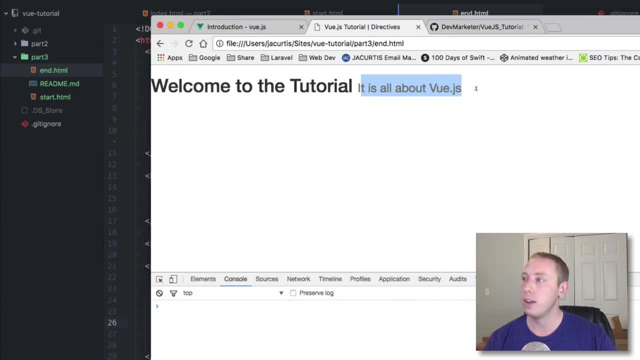 over and, sure enough you can see, it says welcome to the tutorial. It's all about viewjs, All right, so it actually inputted this small. Let's go and inspect the element real quick and you can see that inside this h1 right here, we've got the text. and then it inserted the small tags and this is. 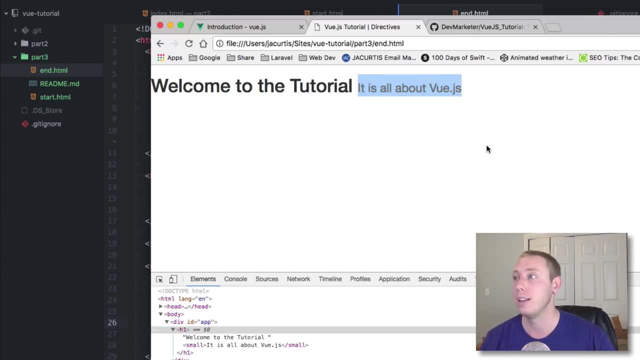 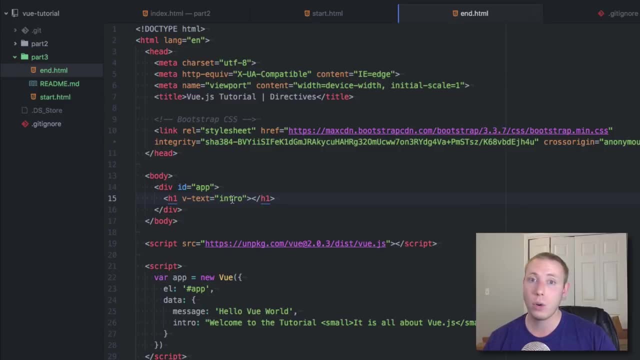 what the small text does. This is because we pulled in bootstraps, so we have this functionality. Now you might be wondering if it's any different than v text. Well, let me. let's show you real quick. If you do v text, you're going to find that it actually renders the text directly. So let's go. 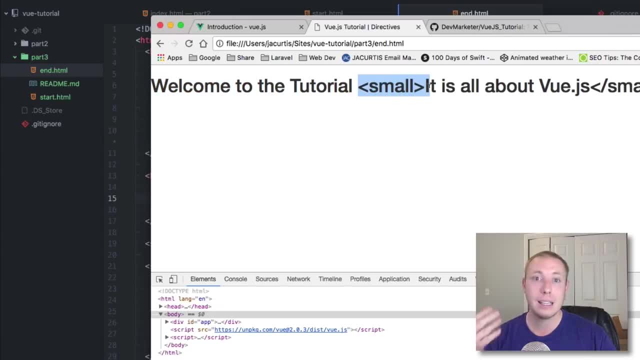 back over here and refresh and you can see that now you're actually getting the text, the actual html attributes, Okay, so this is good to know. if you want to insert html directly, this is the way to do it. Okay, the v html directive. Cool, let's learn about another, a couple other ones, So we 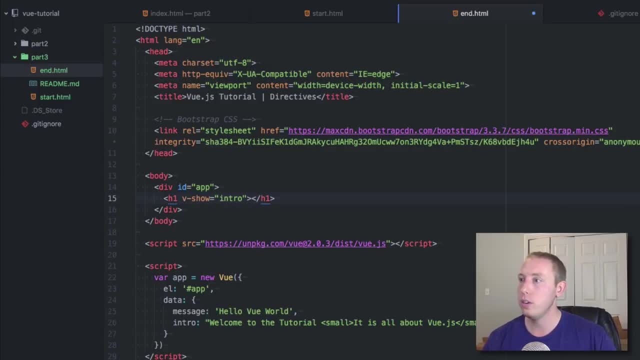 also have one called v show. So let's go ahead and do this and we're going to say: it's another one here, and we're going to say: we're going to call it viewed, We're going to set it equal to true. All right, so, oh, we don't need. 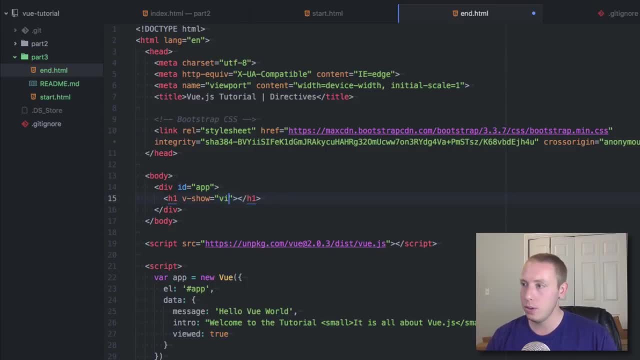 that We don't need that there. Okay, so let's go ahead and set this to viewed and we're basically saying: you have viewed this page, Okay. so this is kind of a weird example, but it's something I wanted to come up with. So again, the v show. 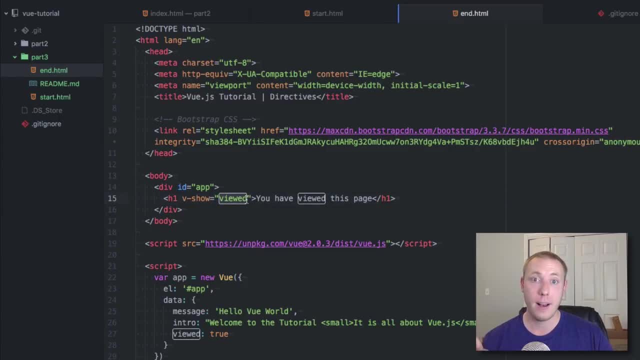 will basically output some sort of. this is basically an operator here. So if anything inserted in here is true, then it will show the element. If it's false, then it will hide the element. Okay, and this actually toggles the css attribute to display: either display none or display. 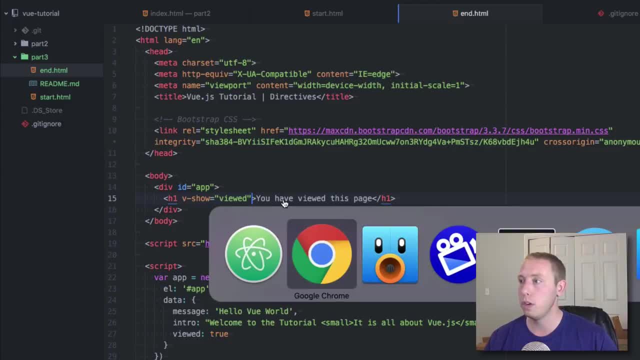 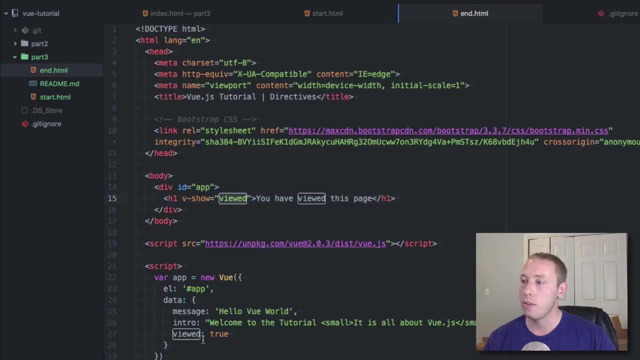 in line, So let's go ahead and just view this. So we would expect to see everything. You have viewed this page and that's because we inserted the text right here directly. However, now if we change viewed to false, then we shouldn't see it anymore. It should go away. right, It goes away. 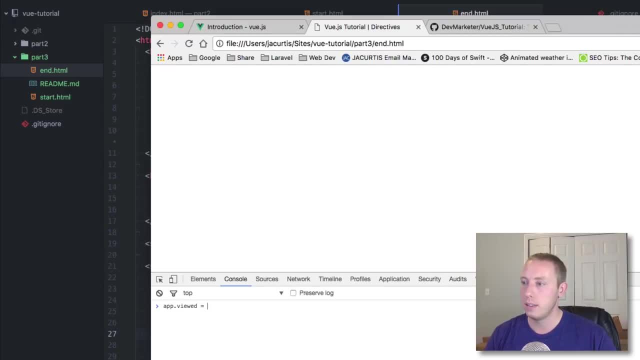 Let's go ahead, just come to app dot viewed and set it equal to true now and we'll. we'll view the the text, All right, and you can see here, if we inspect the element and you can see that we have this h1 here. Let's go ahead and just change it now to false. Okay, now it's no longer being shown. Let's. 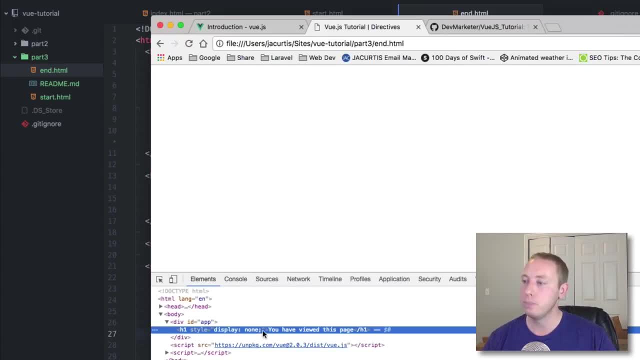 go back over to the html, You can see that it actually is still visible, As you can see here. it's still in the html, but it's not visible. Sorry, I said it was visible. It's still in the html, but it's not visible is what I meant to say, because it has a display, none attribute attached. 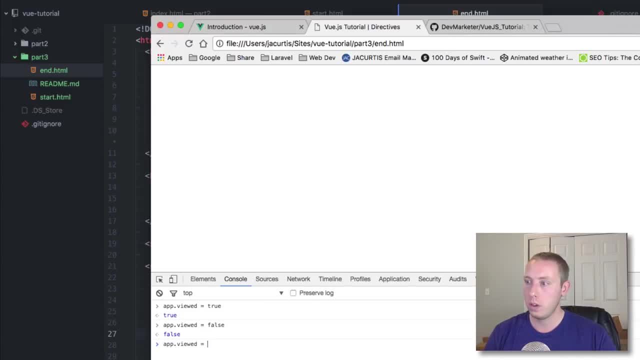 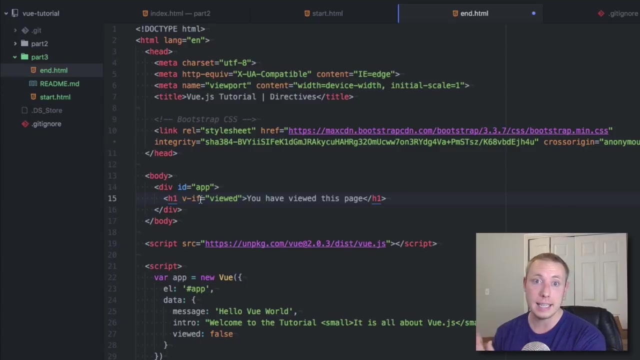 to it. Okay, if we set this now back to true, then all of a sudden it's going to, it's going to show it, So it gets rid of that display. none All right now. the next one that I want to show you. another directive is this: view if and with view if, it's almost the exact same thing as view show The. 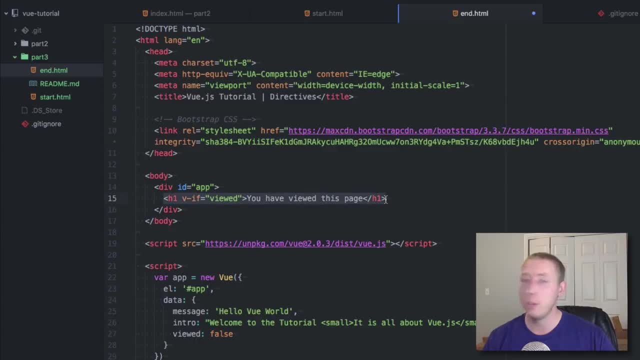 view show actually pulls this. it actually pulls this element in or out of the dom, Okay, versus just hiding it or showing it. It actually removes it from the dom. So let me show you this real quick. We're going to go ahead and save this example. We're going to refresh. Of course it's. let's see. 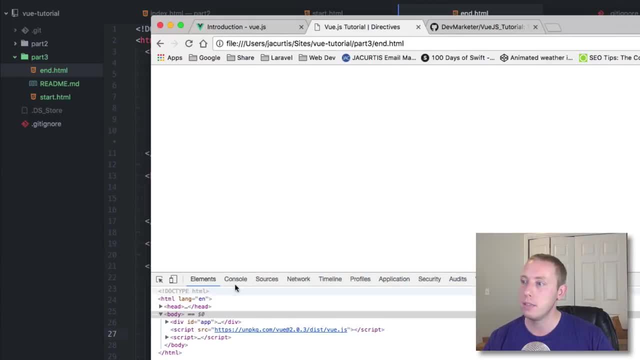 where we set defaults. We were set to false, So it doesn't. it's currently hidden by default. Let's, and if we look at the text here, you can see we've got inside of our div. we've got nothing, All right, so this is the closing of the app. There's nothing in our html here. If we go ahead and 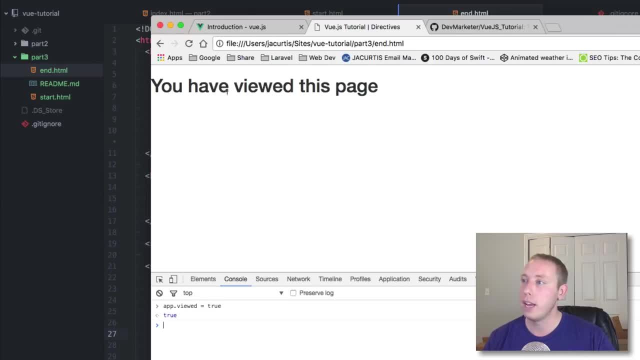 set this equal to true. Okay, now we can see the text. Let's go over to element. and now it's actually inserted the element into the text. Okay, so that's what view if or v, if does? is it actually removes or shows that element, depending on? you know something in the text, So something. 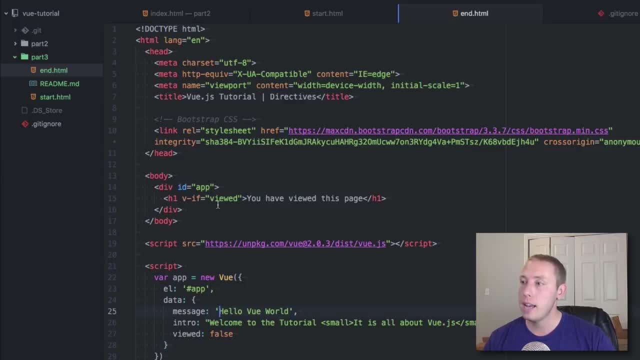 else that we could do is: let's go ahead and let me just show you real quick that you can do more than just put a true or false, a boolean value, in here. Well, it still needs a, it still needs to have a truthy or a falsy value, but you can do more complicated. I'm complicated in quotes here. 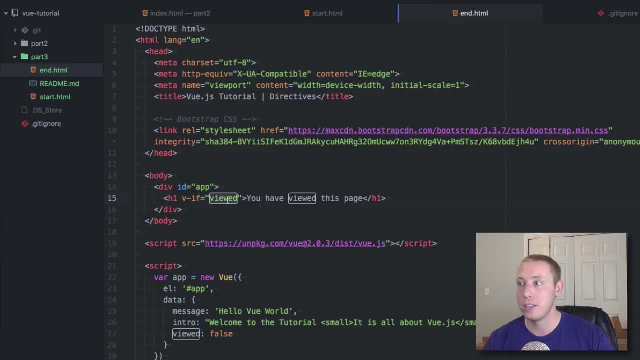 but you can do. you know more advanced operators than just having the element here, So you could do. viewed two is equal to true. Okay. so now we've got two different parameters here. Let's go ahead and say v. if viewed is equal to viewed two, Then it would show the element. Okay. so let's head back. 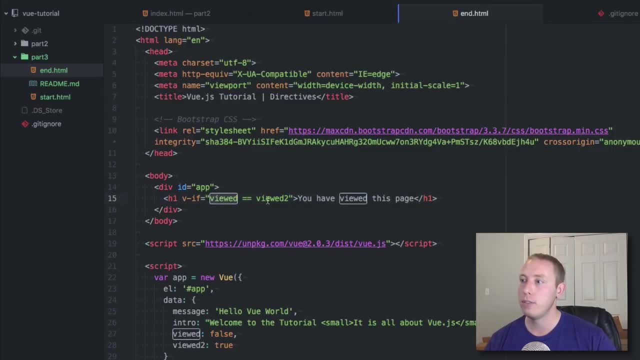 here We don't see the element. That makes sense, because this is saying: if false is equal to true, then it would show it, which it didn't, So then it doesn't show it. So let's go ahead now. let's just change this to: in fact, we can do it in in element here. So now let's go through to our console. Let's 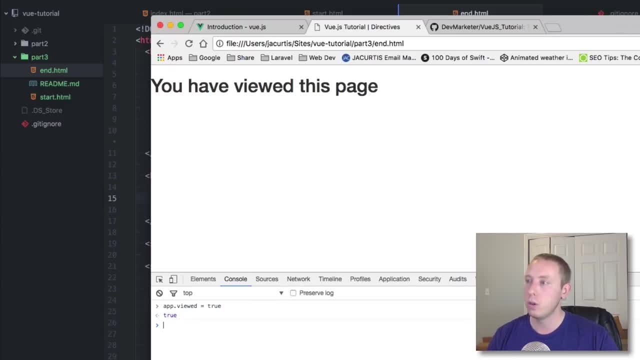 say: app dot viewed is equal to true. Now they're both equal to true, So now it shows it. Okay, so you can see that you can actually do more. You don't just have, you can actually create operators inside of their operating statements, just like that, Okay. 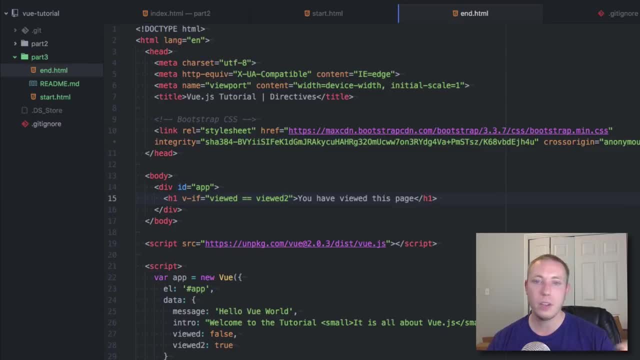 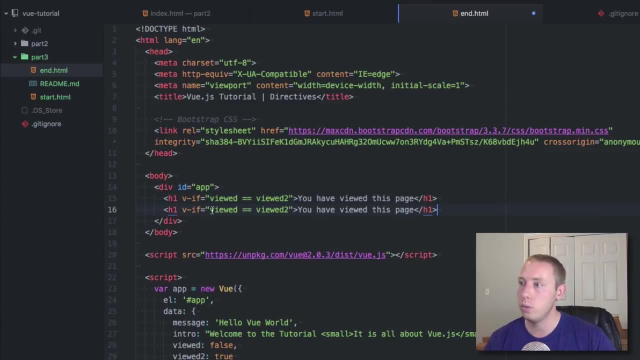 so just kind of showing you some more of the different things that you can do. There's also a view v else. So, for example, let's go through here and let's do v else and let's just get rid of these. Okay, so we've got. so if viewed is equal to true, that in fact we don't need this. 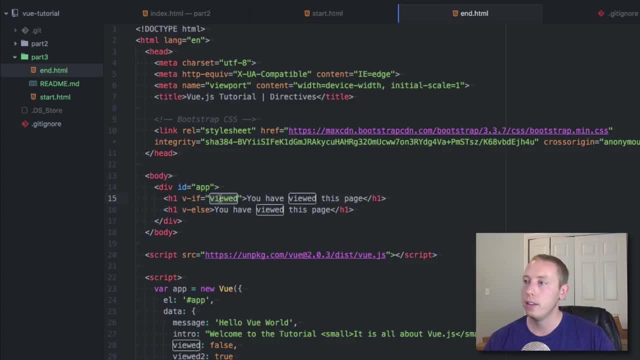 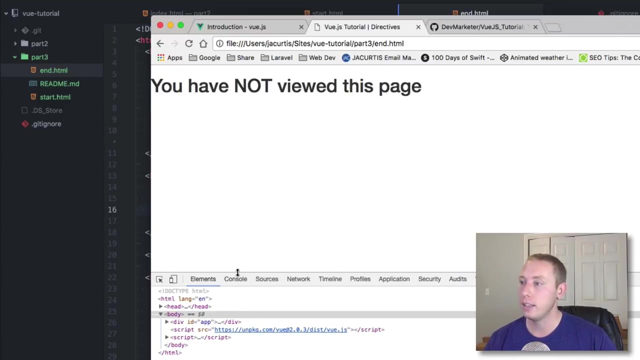 If it's equal to true, or if this is true, then we will show this. Otherwise, we'll show this. So you have not viewed this page, Okay. so now let's go back over here. It says you have not viewed this page because it's false. So now let's go back and let's just change this to true. app dot viewed. 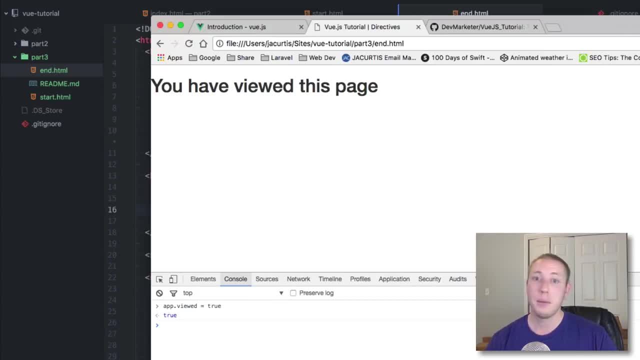 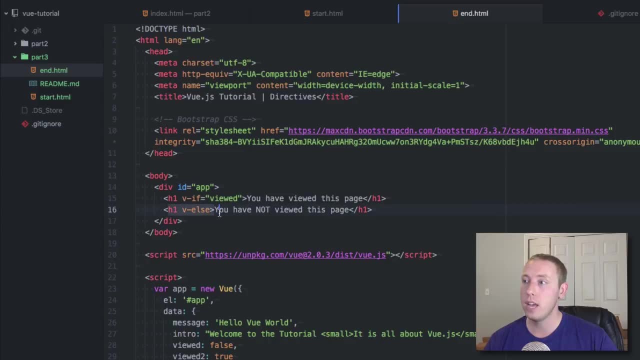 is equal to true, And now we have viewed the page. Okay, so you can kind of create an if or else statement inside of here using these two directives. Now, if you do v, It does require that you have a VA. if above it. Okay, so you have to have both of these here, have to have to exist, All right, so that's VV, else. 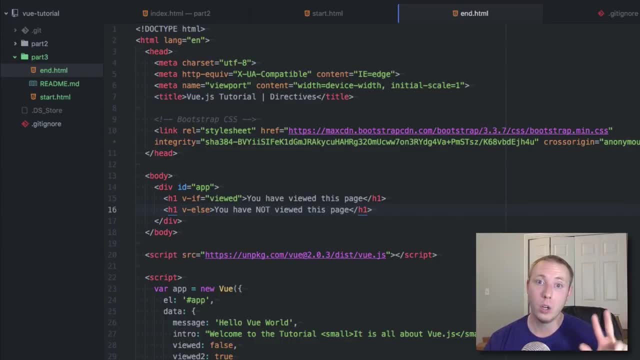 We also learned about V show. You can also do things with loops, which we'll talk about in the next video. and then there is You can also use directives for handling events, which we'll talk about in a future video, and you can use the directives for binding. 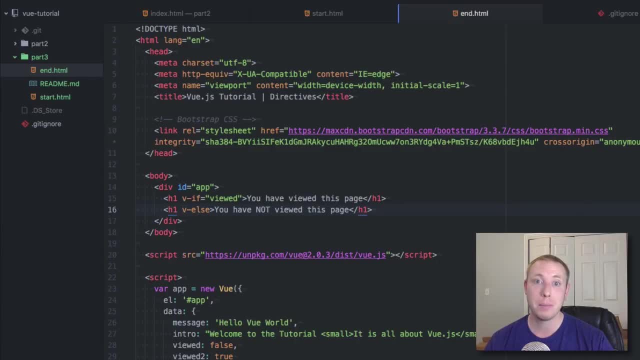 Okay. so there's lots of other things to do. I kind of want to show you some of the basic ones in the video today, But you can kind of see that these directives are like little functions that you can add super, super easy. So you have all this really advanced functionality. That's basically by adding V if V else 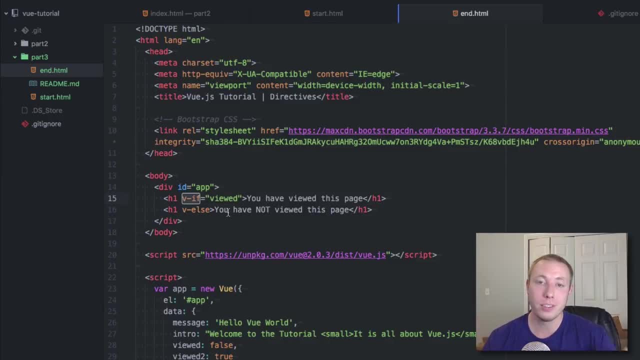 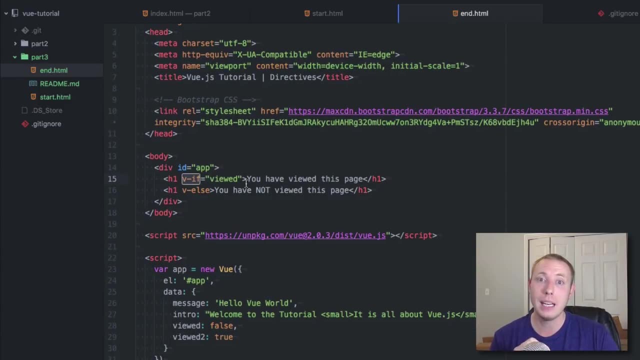 You have all this like advanced functionality that you're writing almost no JavaScript, but it's all powered by JavaScript. That's where view starts to become powerful. now You haven't seen it yet, But we can actually start binding these two interactive elements and that's what it really gets powerful. 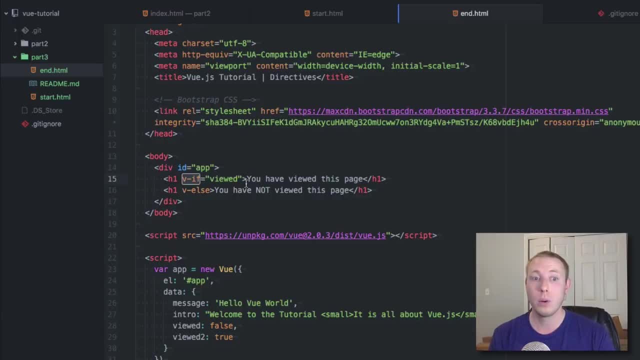 Once we start seeing the two-way binding in place, That's when you're really gonna start seeing The power of view. now, before we finish the video, I want to show you a couple of the other ones that are kind of simple, the other Directives that are simple, and then we'll be done. So let's go real quick here. I'm gonna go ahead and just 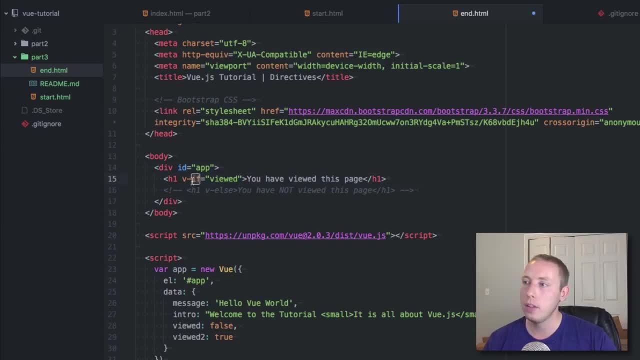 Comment this out and let's go ahead and take a look at a couple of the other directives. So now another thing you can do is that you can actually tell it. for example, Let's say that you wanted. Let's say you had brackets in here and you wanted to output message right. 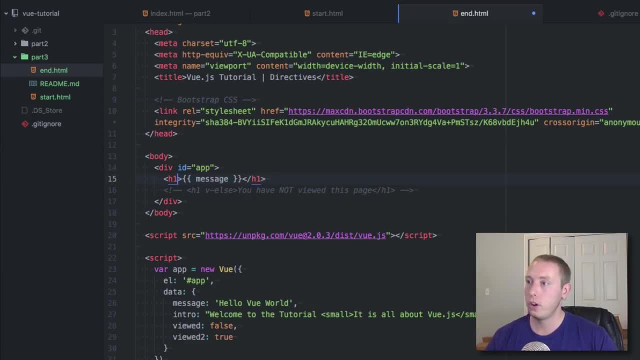 Okay, so we know that this will Currently show the value of message. right, Let's go over here and just refresh. we see the value of message. Okay, Now what if we actually wanted to show these brackets for some reason? That's where V pre comes in, So we have V dash pre. 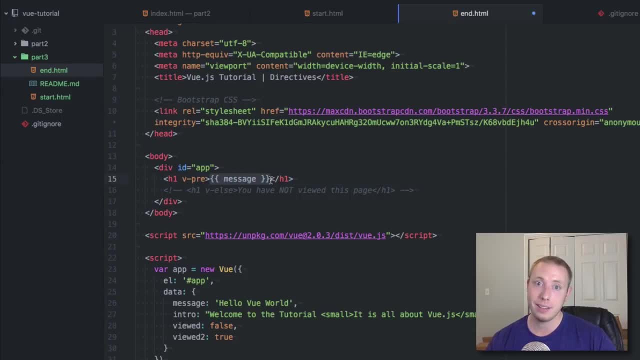 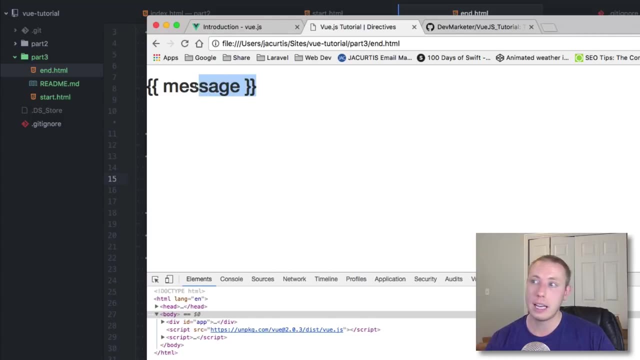 With V back free. it's basically saying: hey, don't render anything inside of here. This is pre formatted text. Let's go back over here, refresh, and now you can see it. actually, you know, outputs the actual mustache tags. It doesn't try to render it, Okay, so that's something else that might be useful. 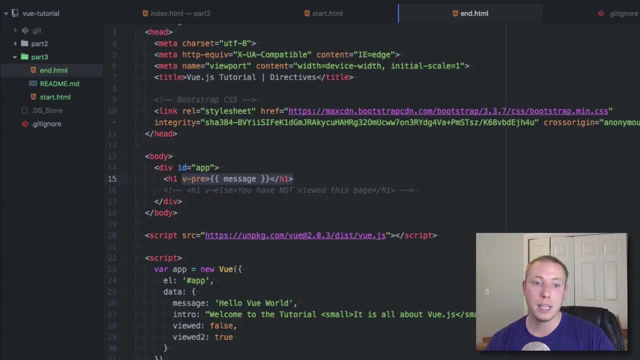 useful that you might want to know about is that vpre. And then let's see, there's two more I want to show you. One is vonce Now with vonce, you're basically saying: only render this one time. Now, vpre never renders it. With vonce, we're saying: render it one time, So let's go ahead and save. 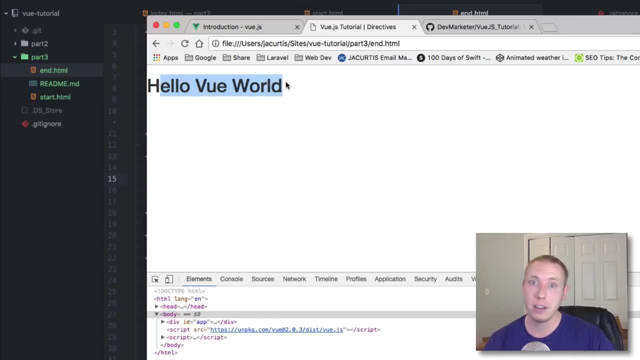 this once again: refresh. It renders it as you would expect. It showed our hello view world. Now, in the past we have been able to change the value of this item on the fly right And you know it would render into the browser and it would update as I change this. But you can see. 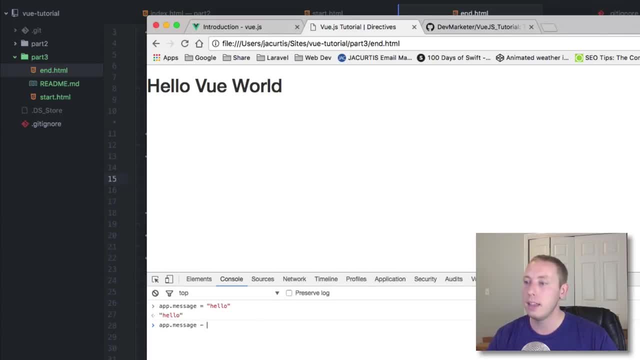 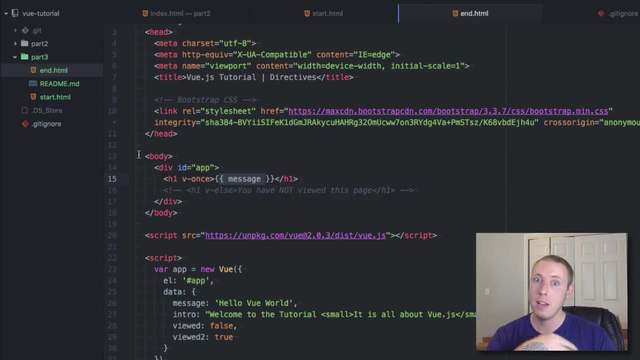 that, as I try to update this, that nothing is happening. All right, keep changing the value of message and yet nothing updates in the browser, And that's because of vonce. You're basically saying, only render this one time And then don't bother re-rendering this anymore. Okay, so that might be something you might want. 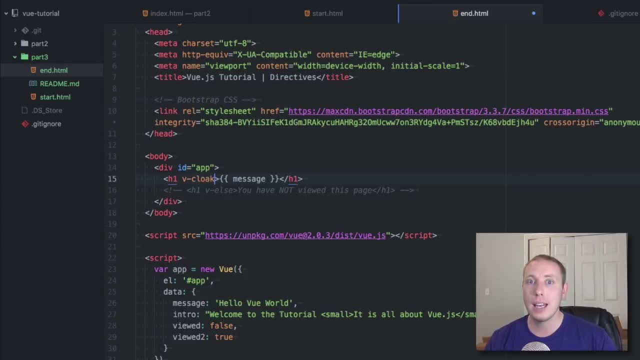 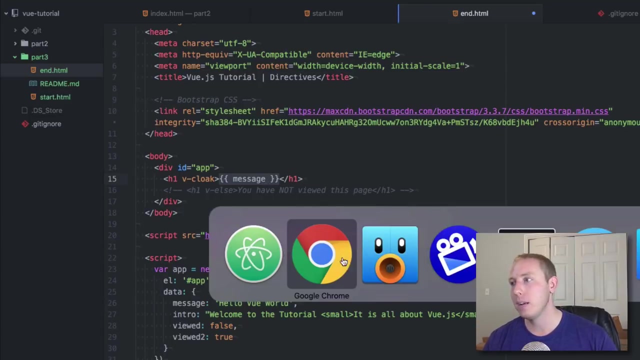 to know. And then the last one is vcloak, And vcloak is kind of nice. This is actually a good one to add to a lot of your directives, because it basically waits to render what's inside of this element until the view has completely loaded. Now it's hard to see on my computer. 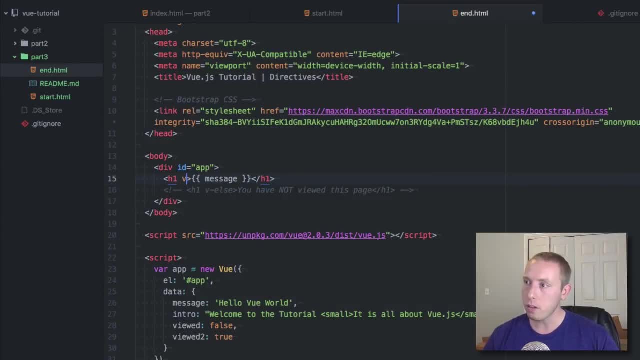 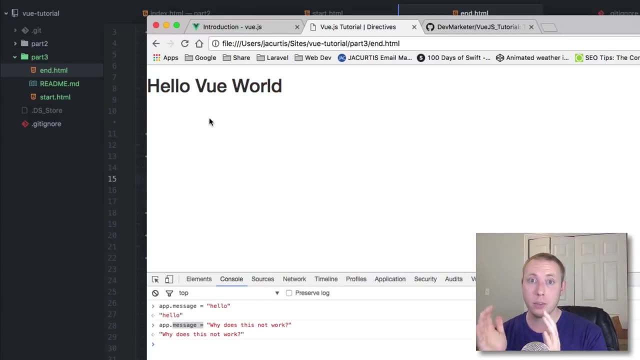 but here let's just go back real quick And let's get rid of this. And if you guys watch really carefully here, maybe I'll be able to slow it down The video. But if I refresh this page you're briefly going to see those mustaches until view. 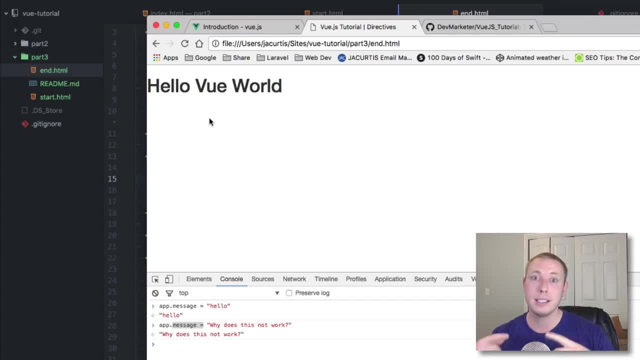 loads the viewjs, loads and initializes and everything, And then it will convert it to the text. right, It'll try to render the text, But there's a brief second there where you actually see the mustaches, So let's go and refresh this And if you saw that right there, you can see how. 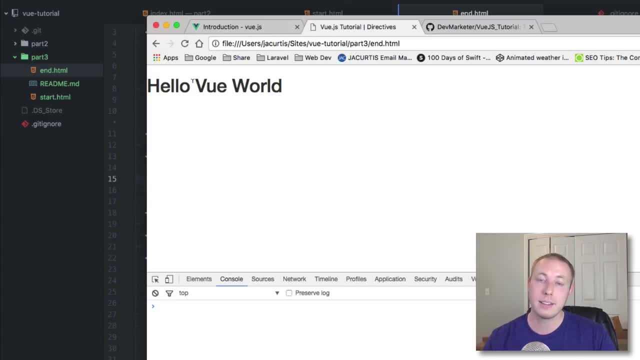 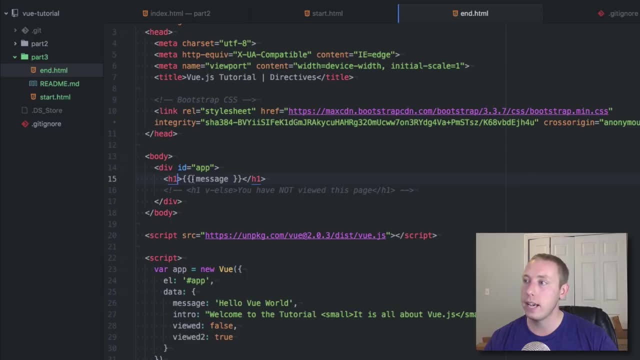 it showed that message And I refresh. You can see that the text is kind of flickering every time I refresh. Let's refresh It kind of flickers That's because it kind of pulls in the actual text here. This is what actually renders at the beginning And then view initializes, takes over. 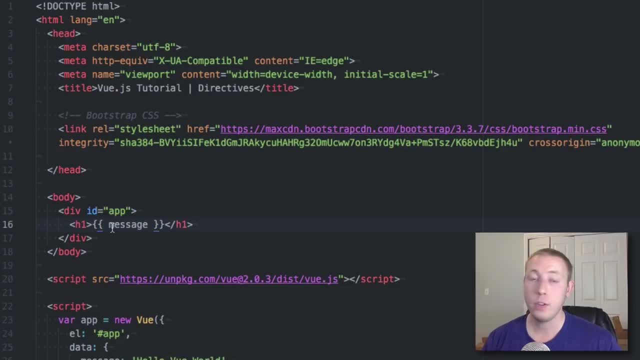 and then updates it with. you know this stuff. Now, if you want to keep that from showing what we can do, is there's another directive called v-cloak. Okay, And what v-cloak does? it's a. 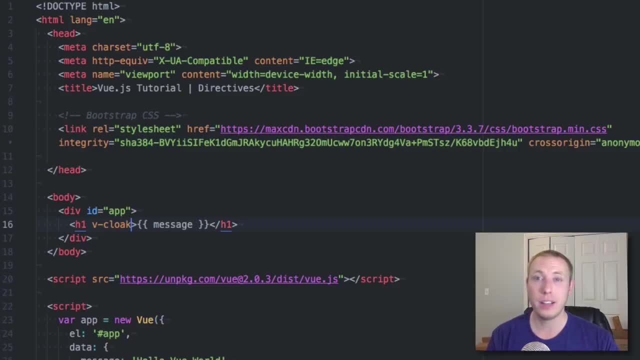 little bit unique in that, basically, v-cloak does almost nothing, But what it, what it represents, is that this v-cloak directive will stay inside of this element until viewjs finishes loading. Okay, Once viewjs finishes loading, it's initialized, it's ready to go and it's ready to. 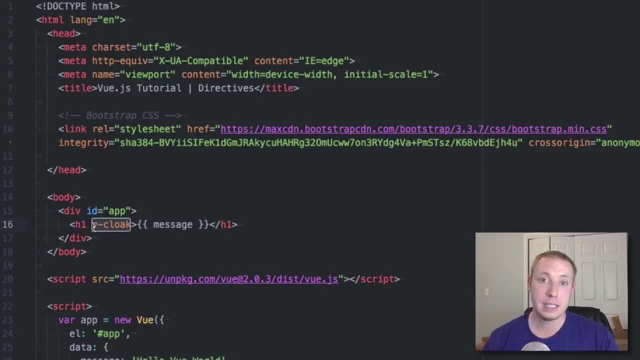 start rendering this stuff, then it will go through and remove any instances of view-cloak. Okay, And you might think, okay, that's weird and random. What do I use it for? Well, this is a good example of what you would use it for is you can actually use CSS to grab anything that you know. 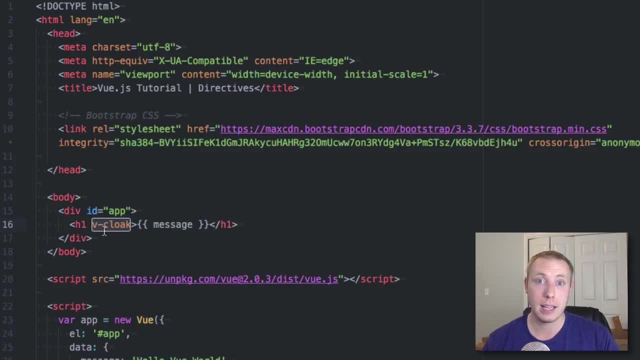 has v-cloak in it and then give it some special styling. Now the most obvious example would be basically to hide it. So this way you don't get that flicker. Everything would be hidden and then, when view has finished loading, then it will just load the. 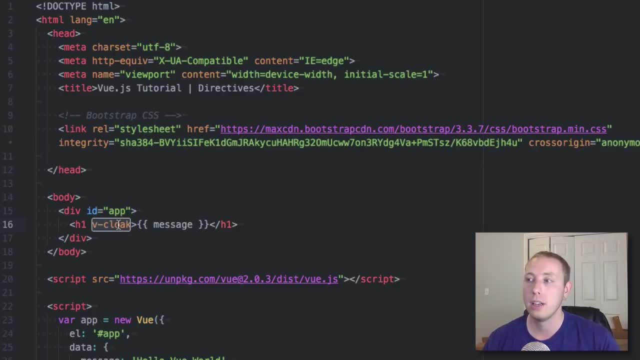 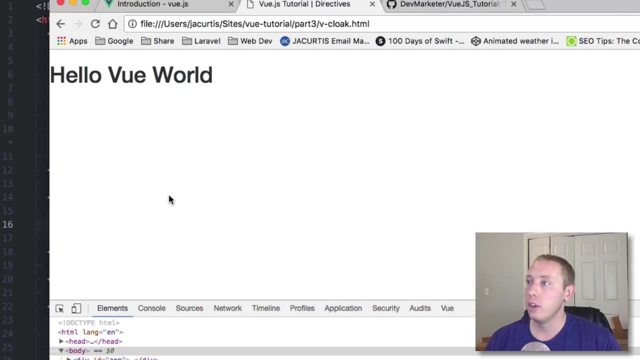 correct element from the beginning. You won't see the mustache brackets. Okay. So let me just show you real quick. We've got v-cloak inside of here, Okay? So, in fact, if we go over here and look at, 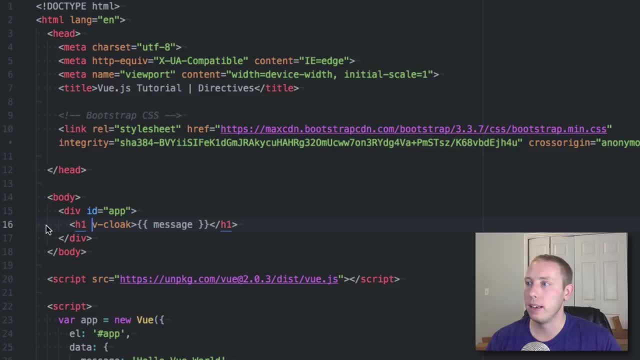 it refresh, you're going to notice that nothing really changes. It's exactly the same way as it's always been. Okay, v-cloak doesn't really do anything. However, you can target v-cloak using CSS, So let's go ahead and do that here. Let's do some style tag up here at the top. 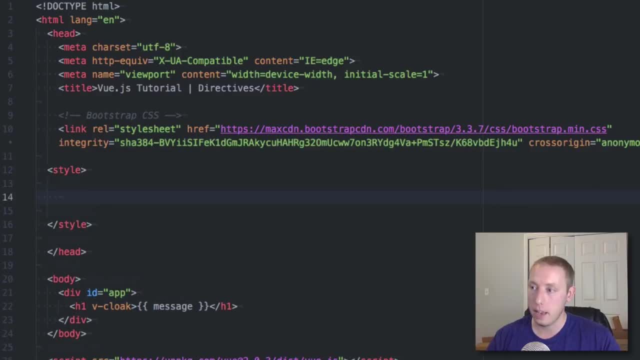 Sorry. And then, inside of here, we can add some CSS. So what we're going to do is we're going to add, we're going to target anything with v-cloak in it. This is any element, Of course, if you. 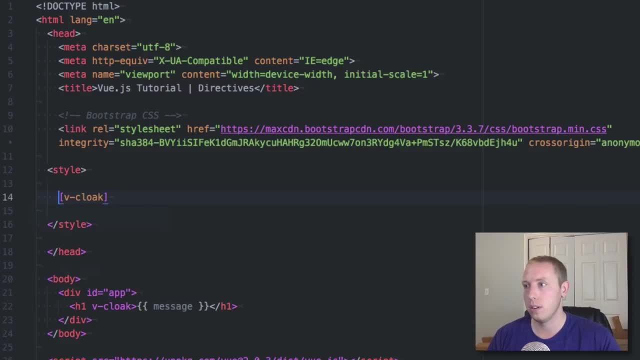 wanted. you know, only divs you could. you could do that, But we're going to target any element with v-cloak and we're going to give it a display of none. All right, So let's go back over here. 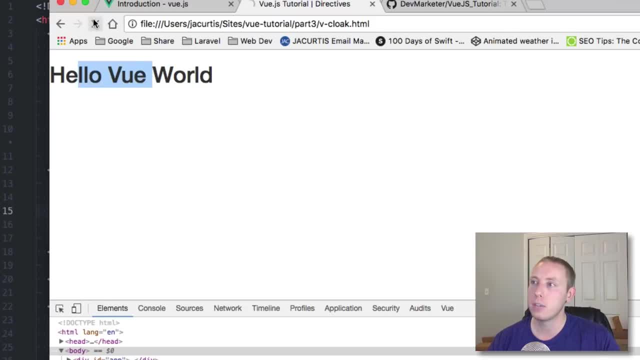 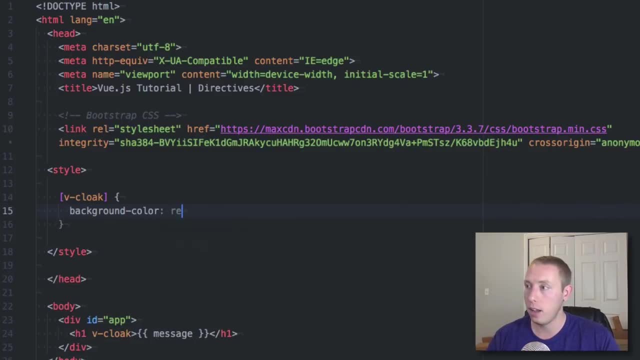 We refreshed. You can see it flickered, but you don't see the mustache brackets in there at all. Now you can do anything with this, So we could also do. for example- this will make it a little more obvious- do background color red And then we refresh over.